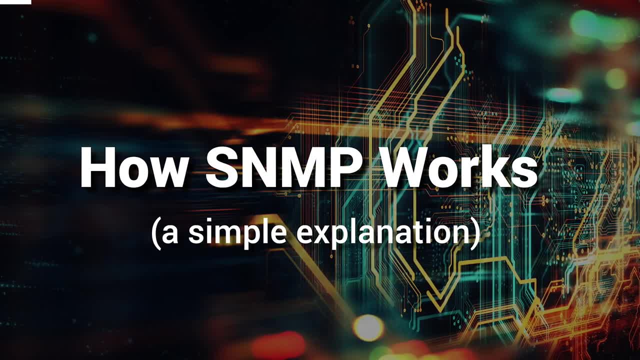 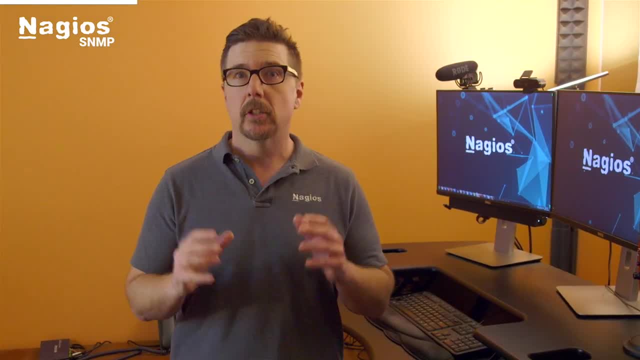 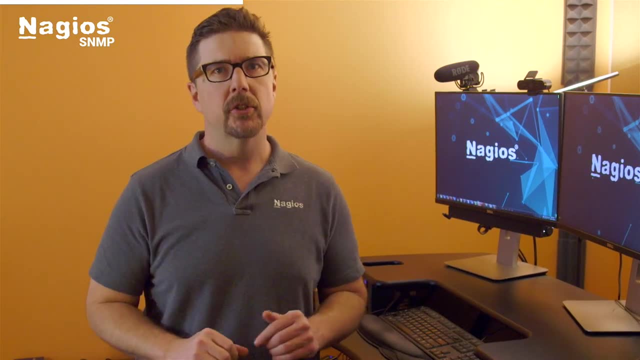 Hey everybody, welcome to this SNMP explainer. In just a couple of minutes I'm going to teach you enough about SNMP to be able to start monitoring devices. While SNMP is a little complex, there's a lot you don't need to know just to start monitoring. So we're going to focus. 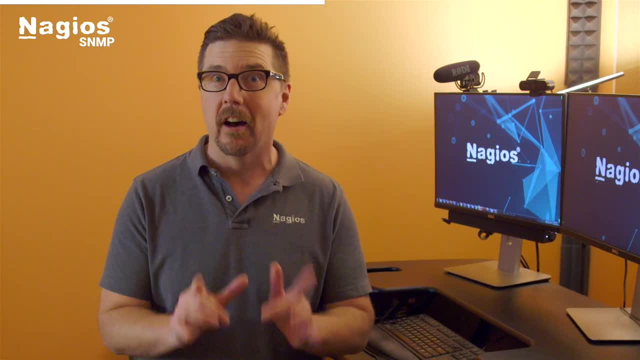 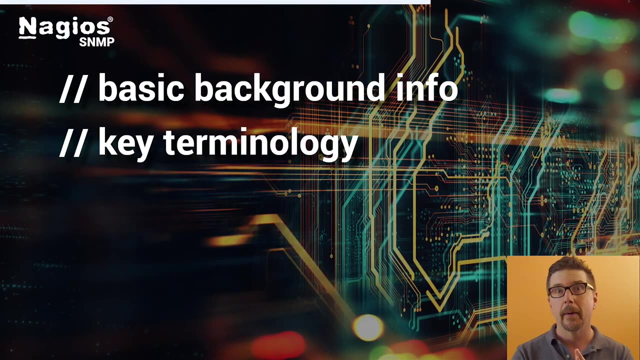 on the absolute basics here and I promise I won't get you lost in unnecessary details. How are we going to do that? Well, we're going to talk about some basic background information. We're going to talk about two key terms you need to know. We're going to talk about why switches. 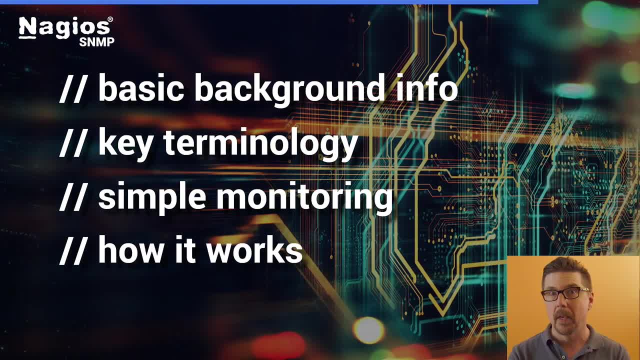 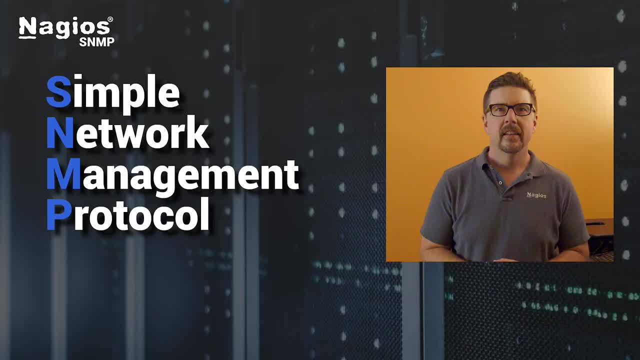 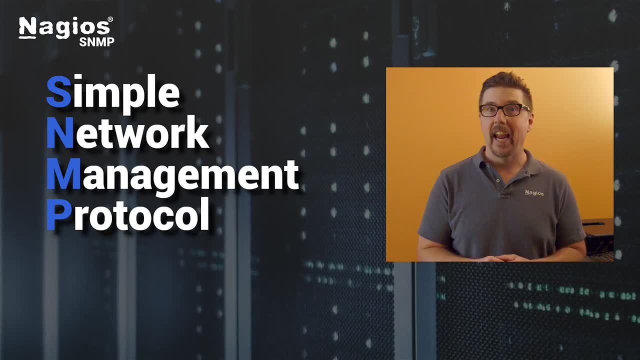 and routers are simple to monitor. We're going to talk about how SNMP works on a practical level and we're going to talk about the different versions of SNMP. Are you ready? Let's get started. SNMP stands for Simple Network Management Protocol. It's been around since 1988, so it's 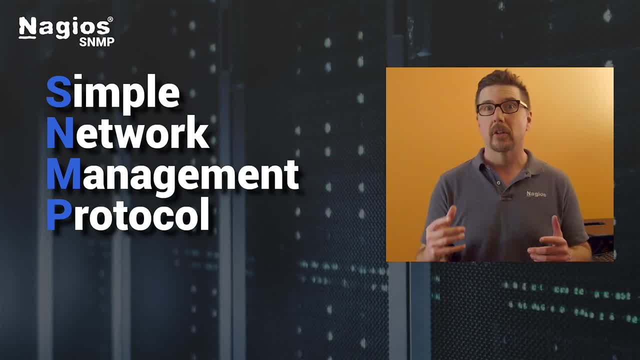 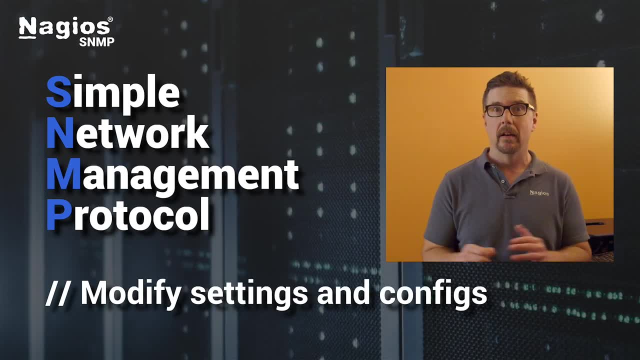 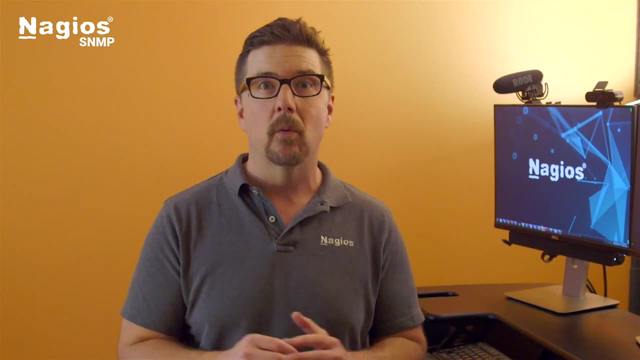 pretty well used. SNMP was developed to allow administrators to both monitor networking equipment's current state and monitor network equipment's current state. It also remotely modifies settings and configurations on the equipment. While SNMP was initially developed for switchers and routers, it has since been extended to a wide array of 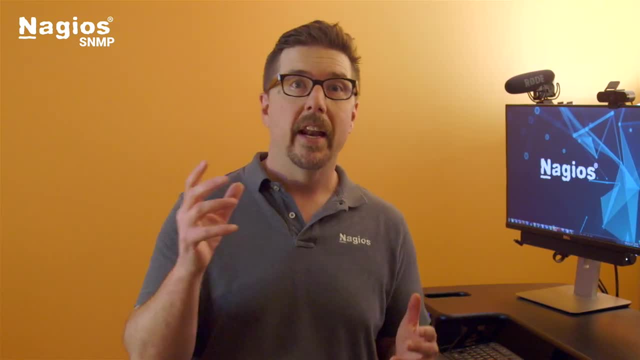 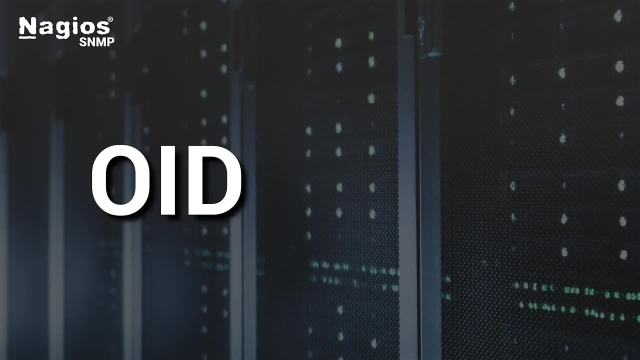 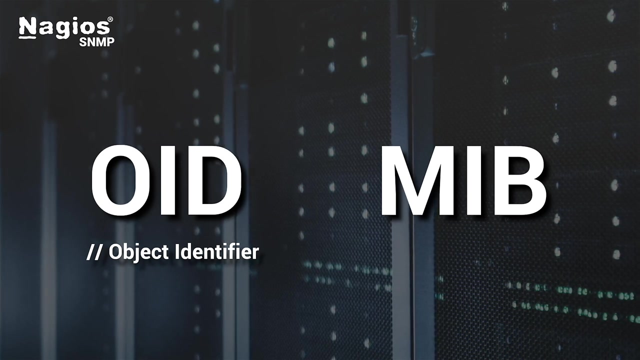 other devices such as Windows and Linux machines, printers and uninterruptible power supplies, among many, many other things. There are two key terms you need to know: OID and MIB. OID is short for Object Identifier. Think of it like this: Anything and everything on a device that can't. 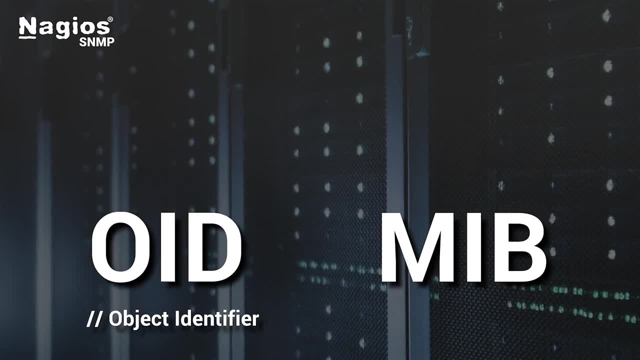 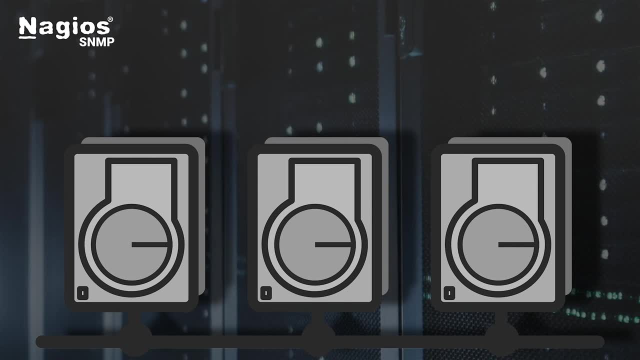 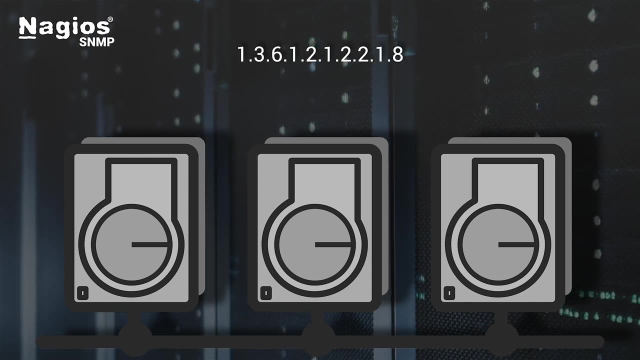 be monitored with SNMP? has an OID, For example? say I want to monitor the temperature on a network attached storage device we have here at Nagios? The OID for the temperature sensor on the device is a bunch of numbers separated by dots. That number might look confusing, but all you really. 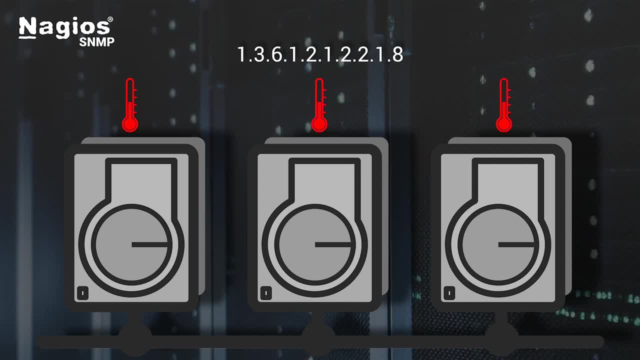 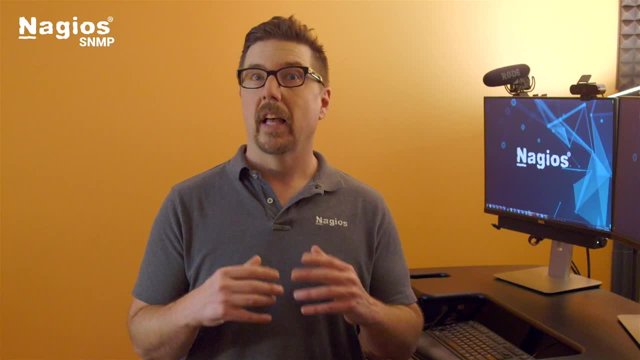 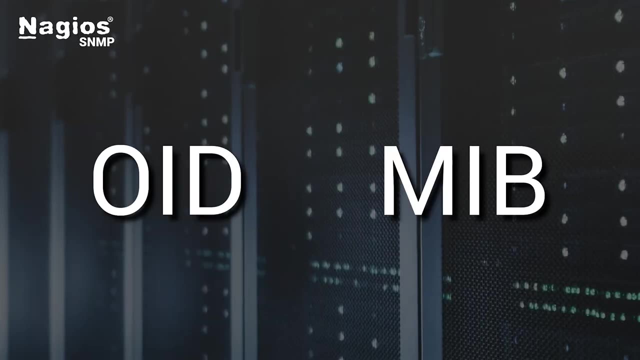 have to know is each thing we can monitor, like device temperature, has an OID. You might think of an OID as something similar to an IP address for a value. We use an application like Nagios XI to ask the device what the value of any particular OID happens to be. MIB is short for Management. 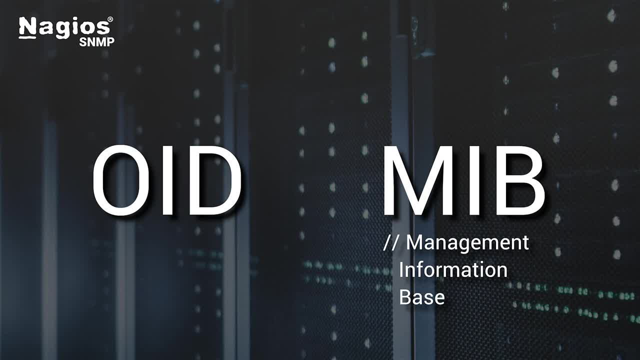 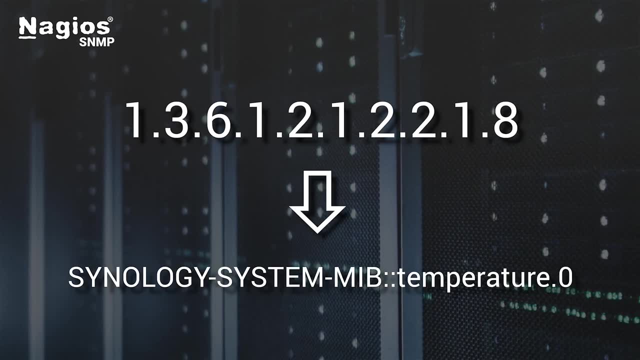 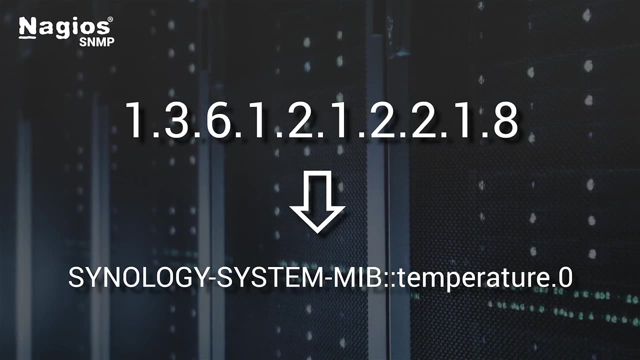 Information Base. That sounds a lot more complicated than it actually is. A MIB is a text file that allows us to translate numerical OIDs into word-based OIDs. So instead of using the numerical OID for the temperature sensor in our example, we can use this word-based OID, which makes it a lot. 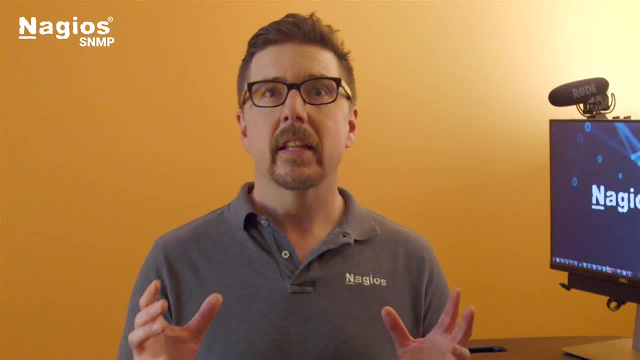 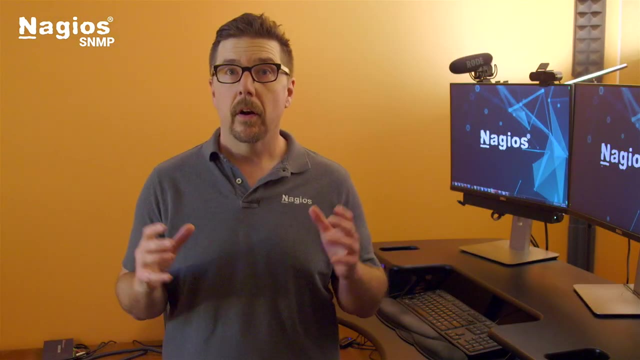 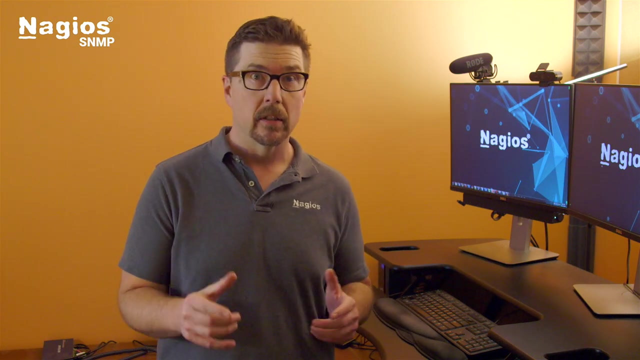 easier to understand what we're monitoring Now. technically, you don't have to use MIBs at all. You can use only numerical OIDs. but MIBs can make your life a lot easier. There are a number of standard OIDs and MIBs that are incorporated into most SNMP implementations by default. For example, on almost 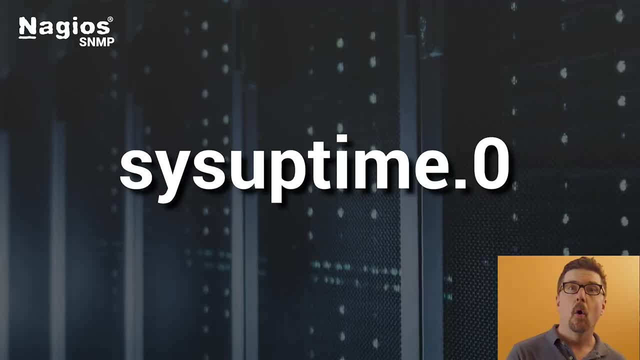 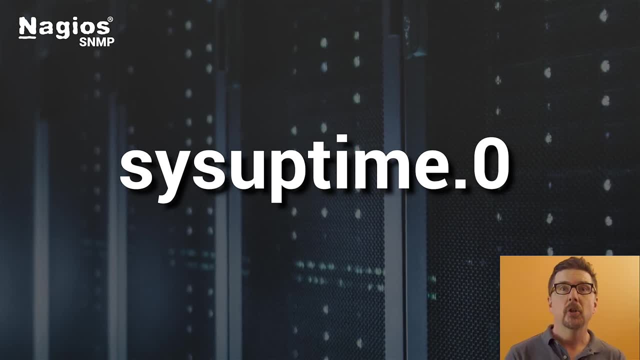 any system out there, you should be able to ask the uptime of a device with the OID sysuptime.0.. This is great because when you go to do basic switch or router monitoring in Nagios XI, you don't need to know a single OID or find any MIBs, because those are already built in. You really only need. 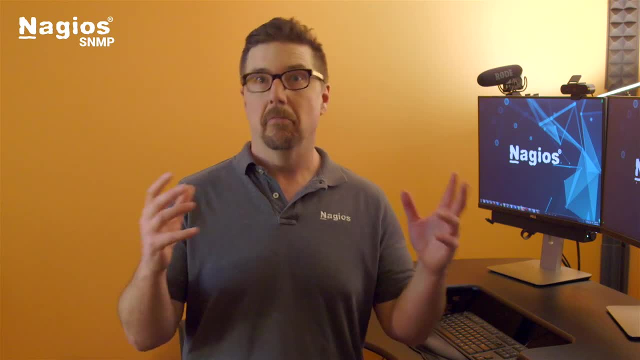 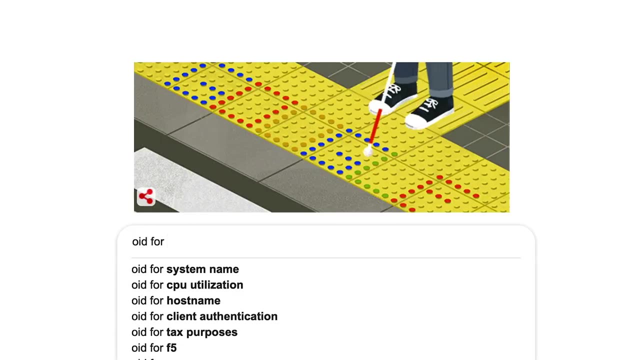 OIDs and MIBs. when you have a non-standard OID to monitor, like the temperature sensor on a network attached storage device, like we just talked about a minute ago, How do you find out what the OIDs are and where do you find MIBs? The best place to start on both of those questions will be the product. 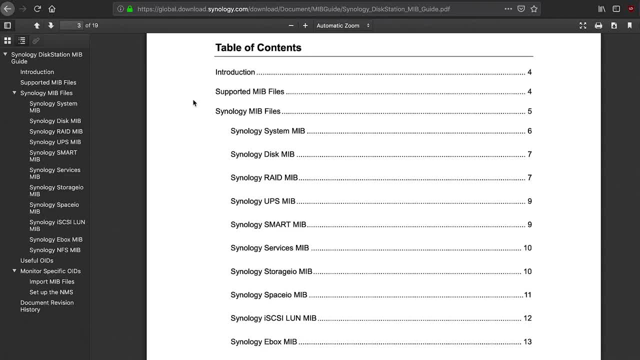 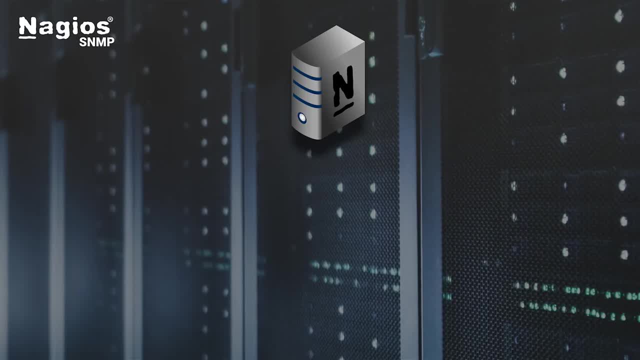 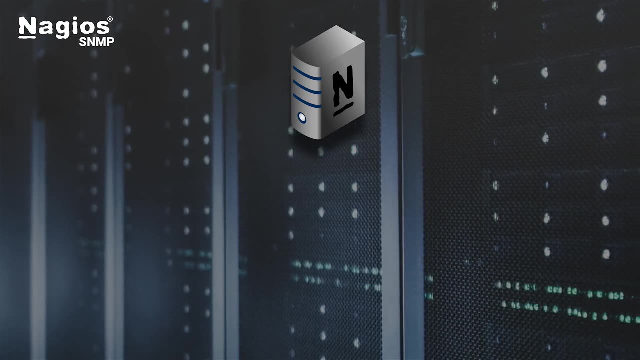 manuals from the manufacturer of the device. Many times these documents are available online and a simple search will get you the information you need. So here is how SNMP gets used in day-to-day network monitoring systems like Nagios. This is what monitors the things you want to monitor. 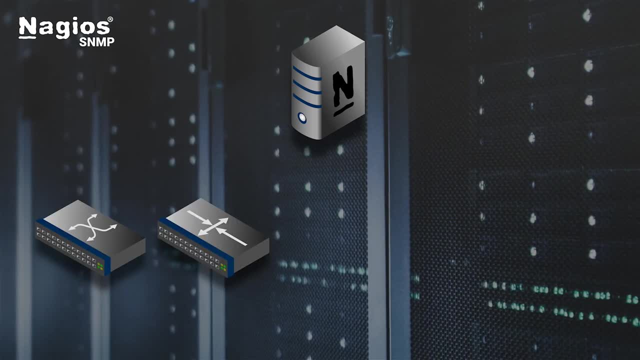 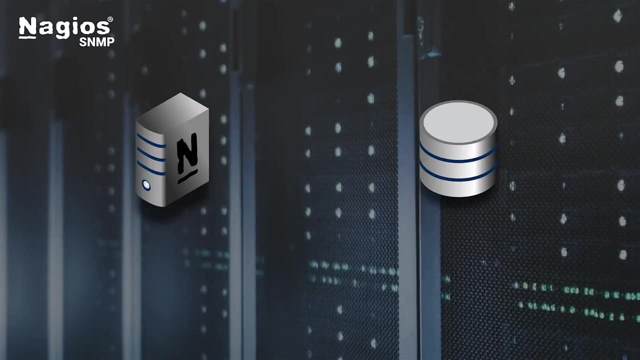 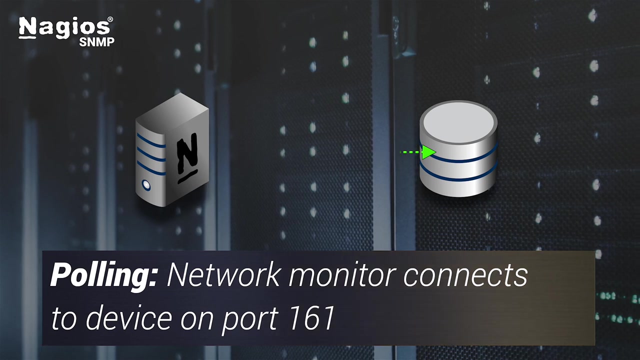 And then you have the things you want to monitor, like switches and routers and servers and uninterruptible power supplies. There are two ways to use SNMP. The first way is called polling. With polling, the network monitoring system connects to the monitored device on port 161 and tells the 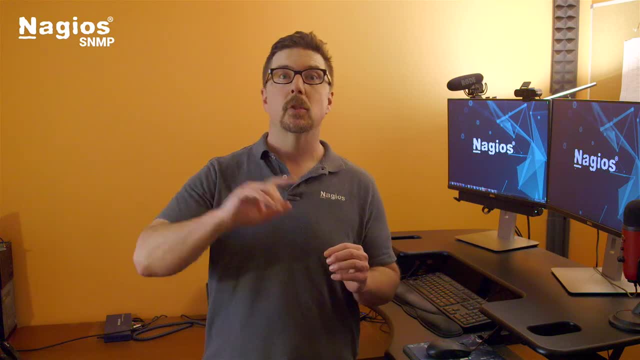 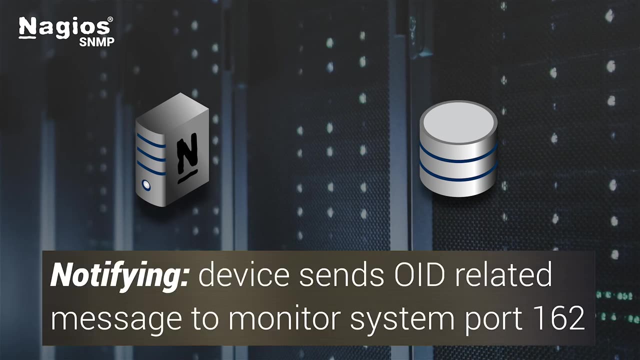 device which OID it wants. information on The device then responds with the information to the network monitoring system's port 161.. In the second way, we do what's called notifying. With notifying, the device simply sends a message about an OID to the network monitoring system's port 162.. 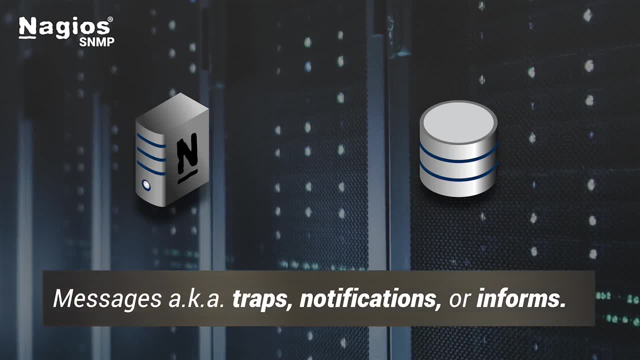 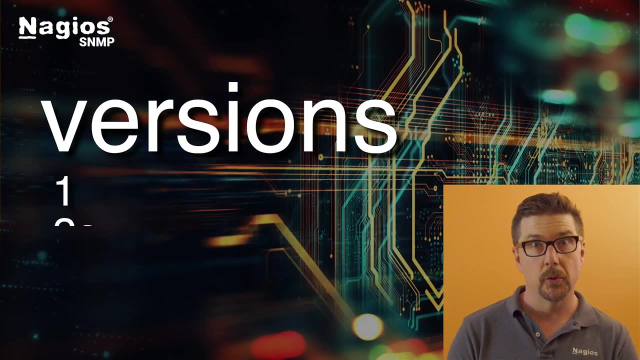 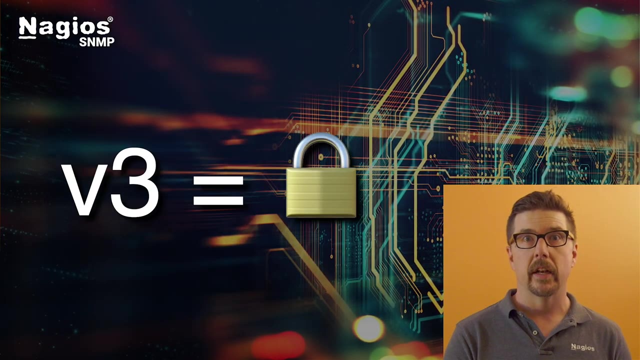 These messages are variously called, either traps, notifications or informs. There are three versions of the SNMP protocol: Version 1,, version 2C and version 3.. The biggest difference for our purposes is that version 3 is more secure than versions 1 and 2C.